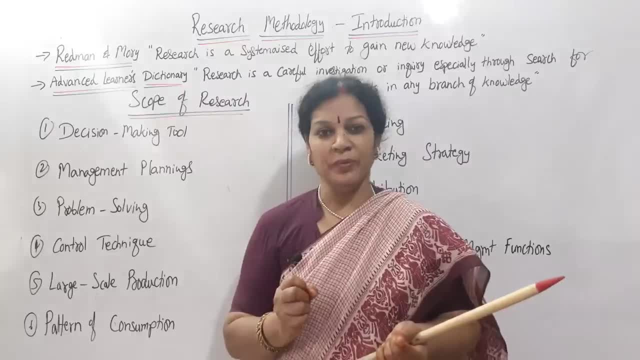 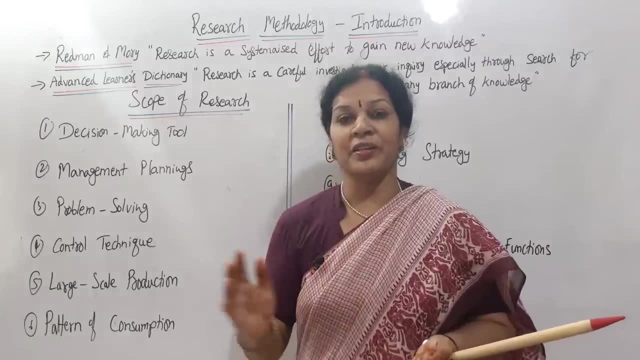 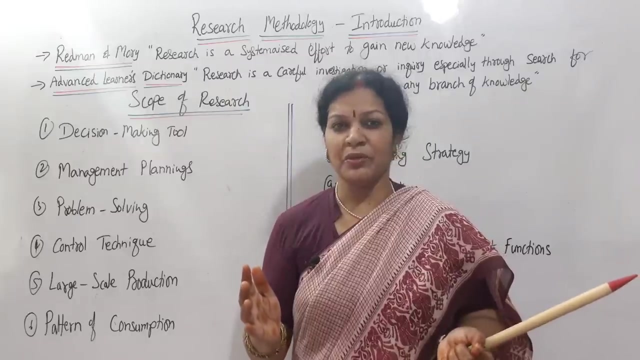 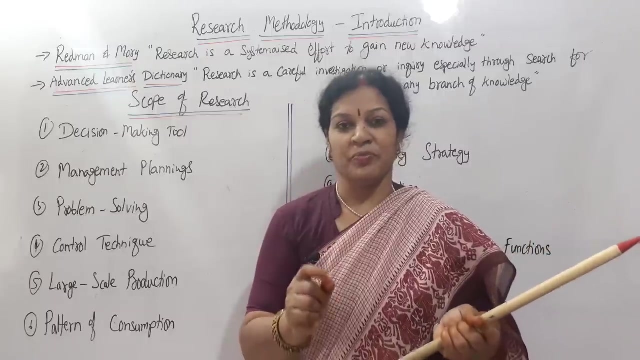 What is research means identifying any problem and analyzing that problem and giving the solution Solution also different alternatives will see. We will be focusing on various aspects then according to that. So which solution would be good? which solution is going to work out that kind of recommendations? we are going to give it through research. So this is especially for identifying problem and giving solution. 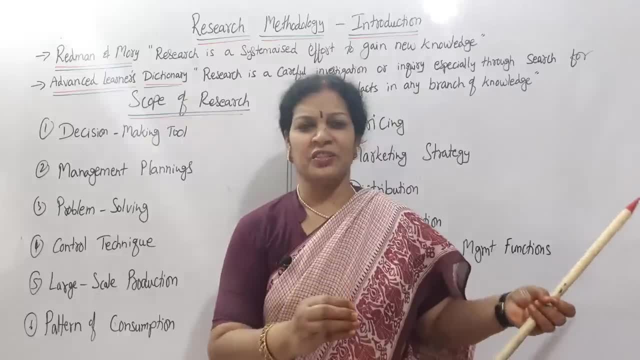 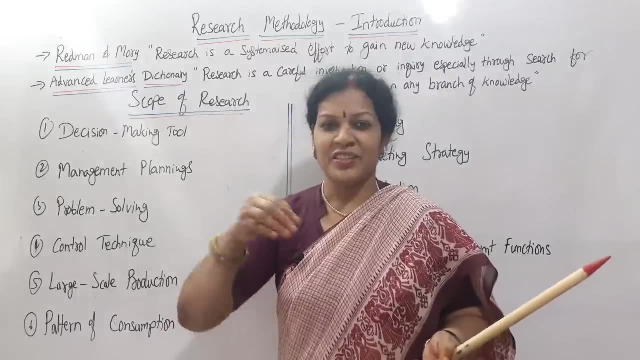 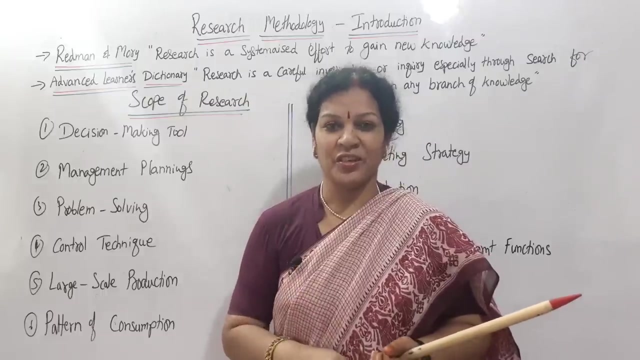 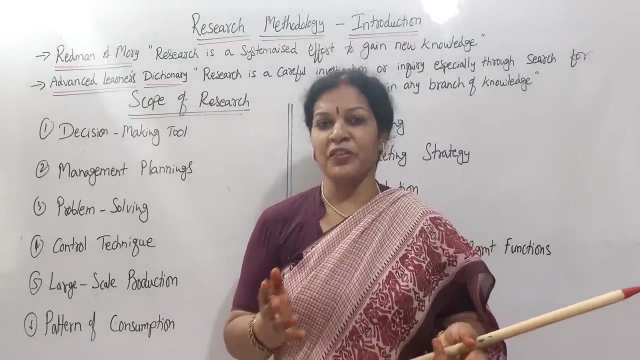 Many people says that research means nothing but search, search, search and you will get somewhat solution. Or in other words, research means gaining the knowledge. Acquiring the knowledge is nothing but the research. Research for many areas, many areas. Especially, when we see our commerce and management fields, We know that marketing is very important. aspect In marketing, research is very important. 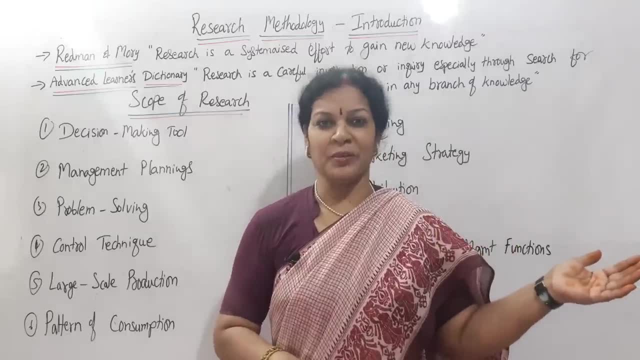 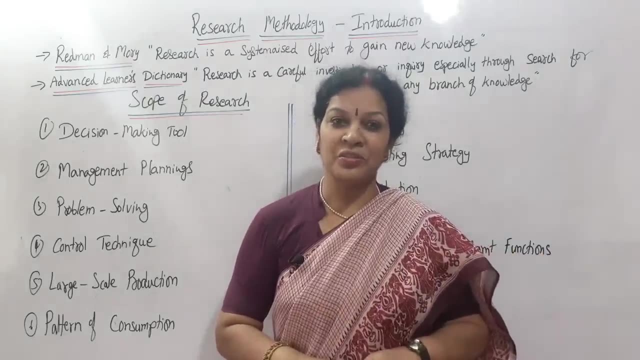 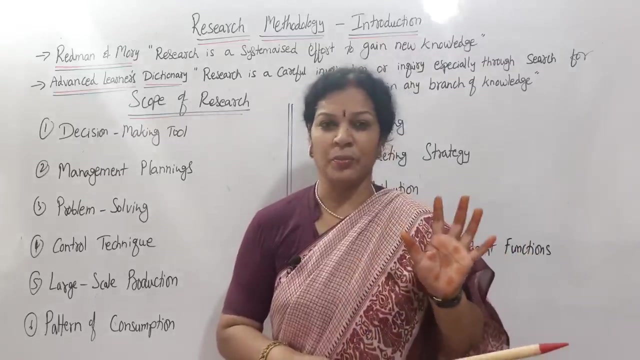 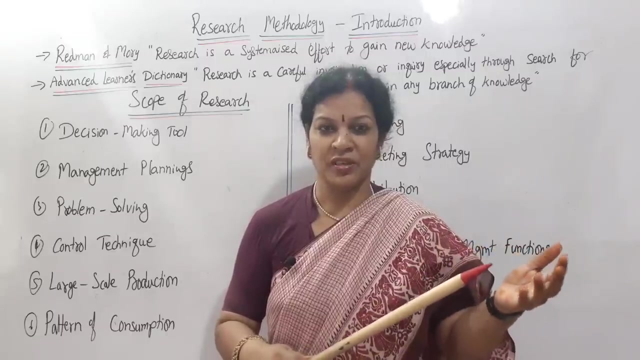 Research is compulsory. Various aspects we can take in marketing. In vast we can enter into the marketing And also finance area also you can do research And in the same way, marketing- sorry, what is that area? HR related also. You can take any kind of topic related to HR, marketing or otherwise finance, any topic you can pick up and you can do the research. At PG level, if you do that topic will be small. At PhD level, if you do that topic will be small. 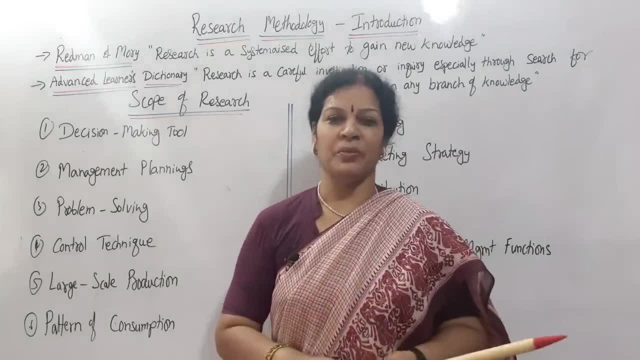 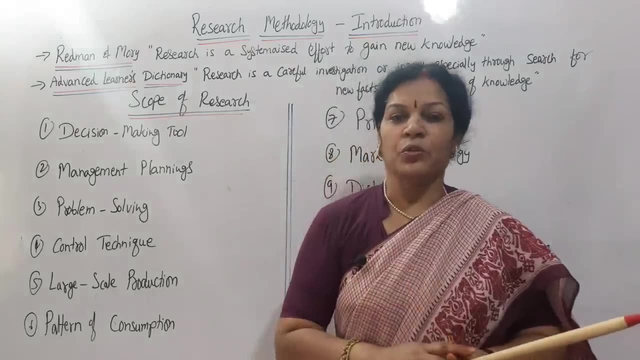 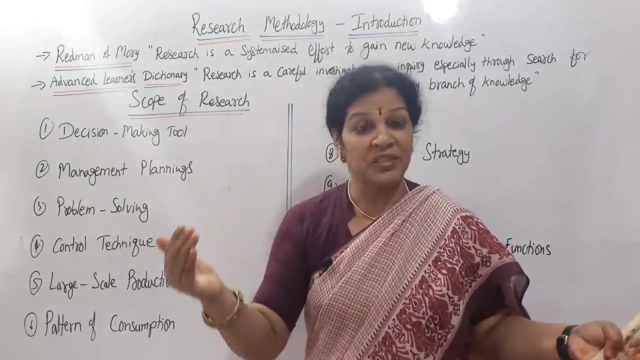 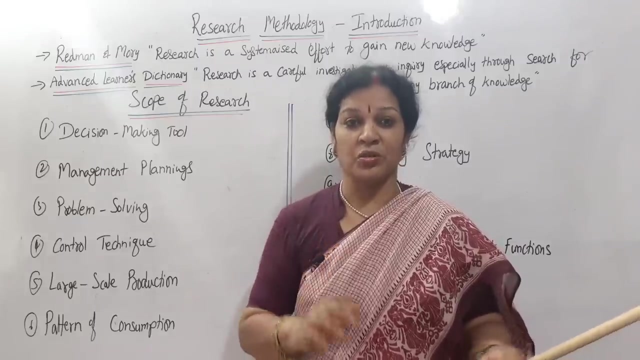 At PhD level you have to go in depth, That's it. That is the only difference between normal project and the PhD thesis. So anyway, so how we can do this research, Whether it is research related to the MBA, commerce or maybe science background students also, they are having a lot of research, They are inventing lot of things through the research. only Process will be lengthy. Sometimes you will say that research is for. 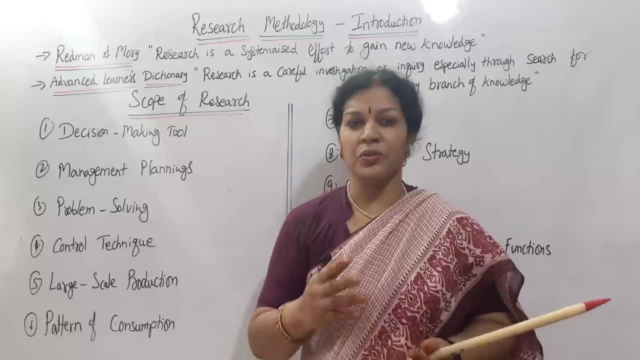 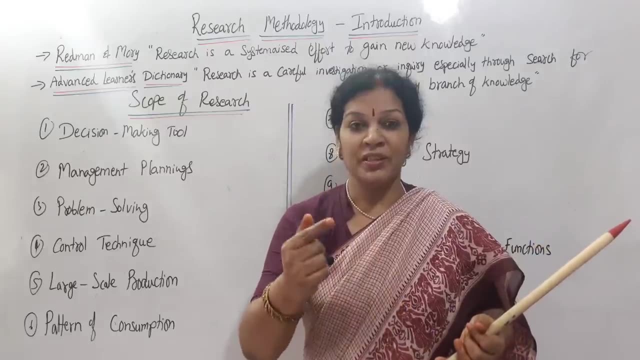 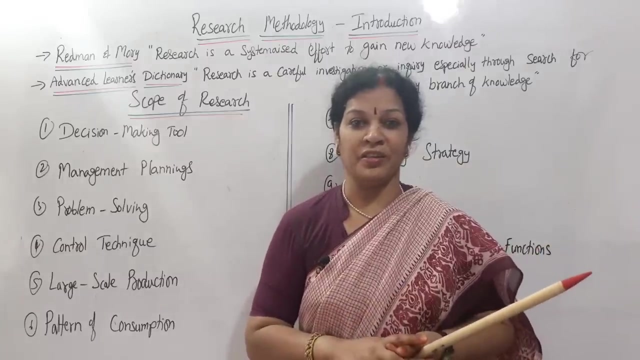 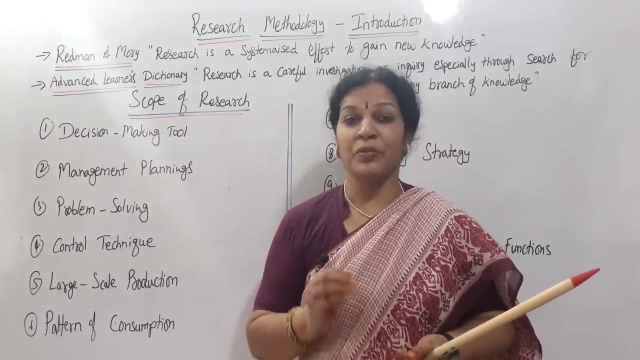 possible and we can complete our research within 2 years, 4 years. Sometimes it may take 10 years, also because it depends on the problem you have chosen And depends on the nature of the problem. Sometimes you may not find a solution. In such cases it will take lengthy period. So, anyway, it doesn't matter whatever it may be, but sincere efforts and having knowledge and working out- These are all going to make a lot of difference. while working out. 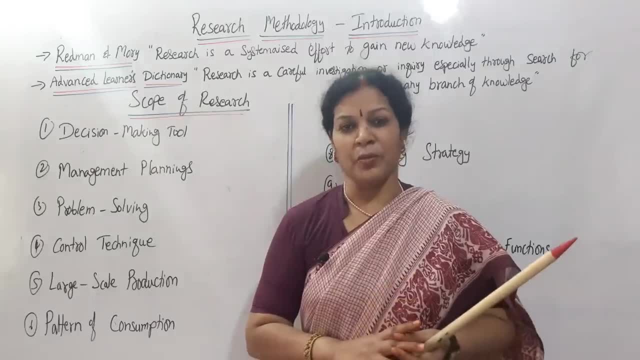 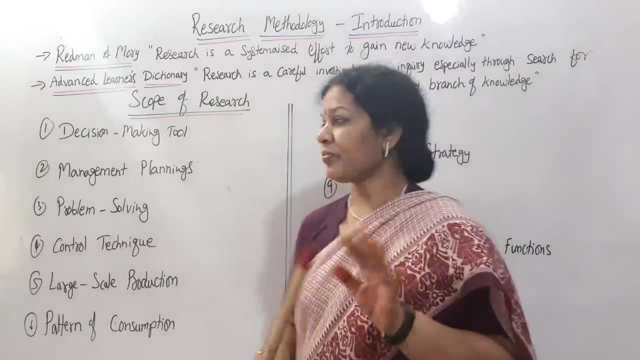 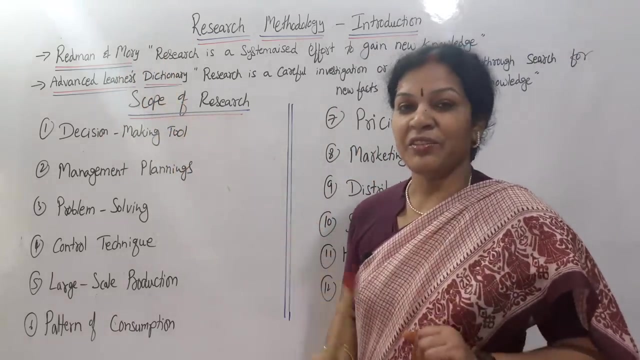 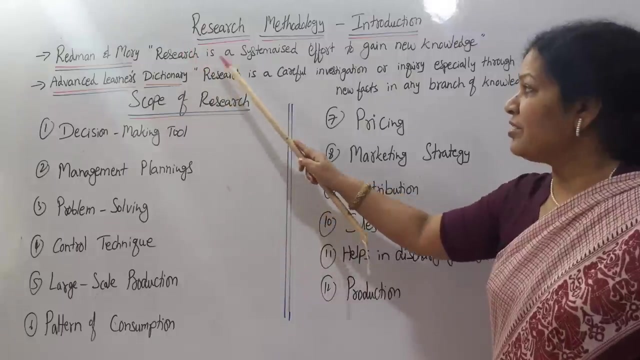 Research on any project or any problem. Now let us see what is the definition of research. Two definitions I have taken: Research methodology. One is that Redman and Murray, Redman and Murray, He has given a simple definition, Easy You will be able to understand and remember. also, Redman and Murray: Research is a systemized effort, Systemized effort to gain knowledge. 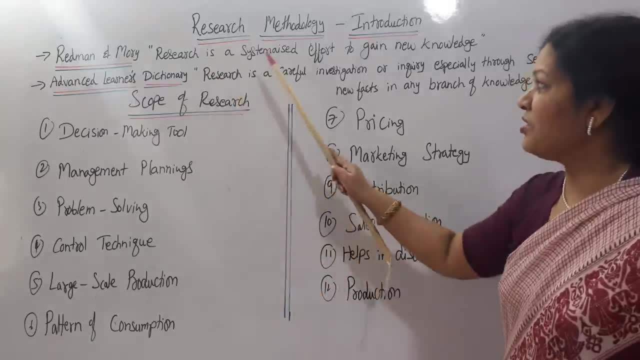 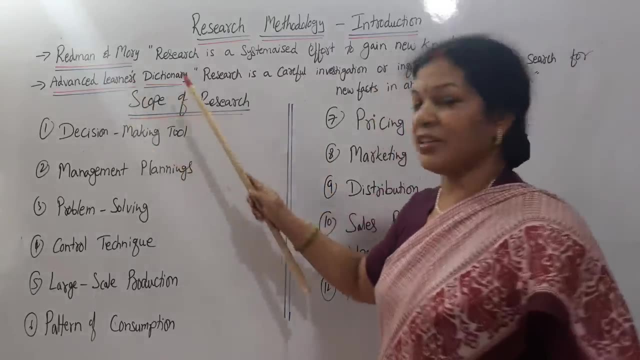 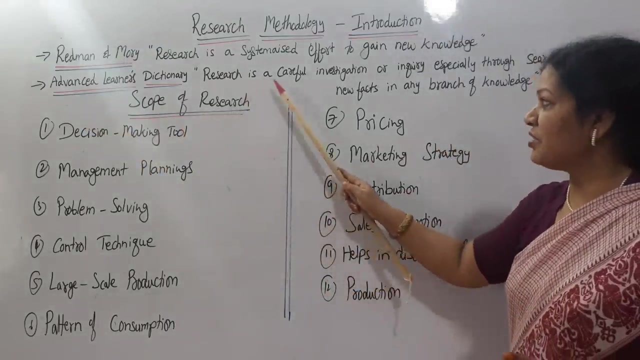 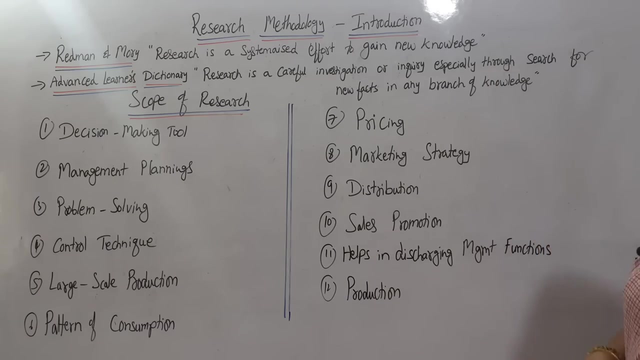 New knowledge Simple. So research is a systematic effort to gain good knowledge. That's all. This is simple definition. There is another definition, that is advanced learner's dictionary. So as per advanced learner's dictionary, this has given research methodology meaning. research is careful investigation or inquiry, especially through search for new facts in any branch of knowledge. Means we are choosing any branch of knowledge, Any specific area that we are choosing. 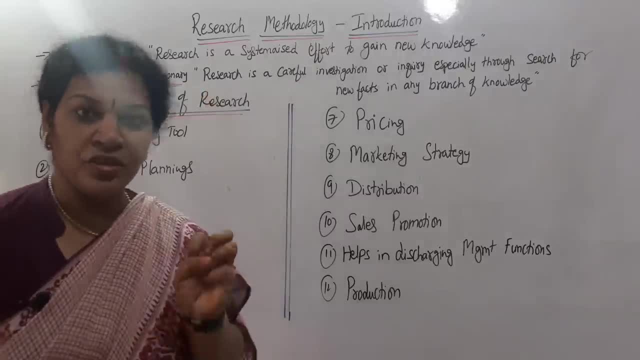 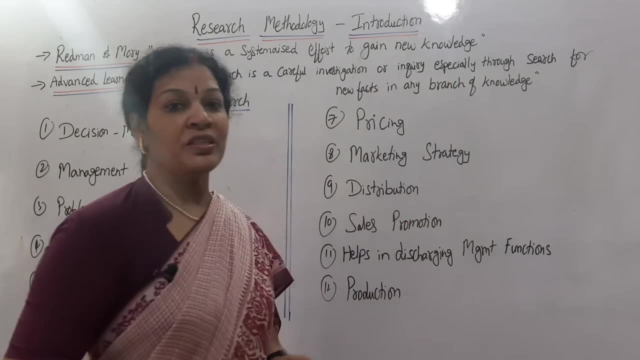 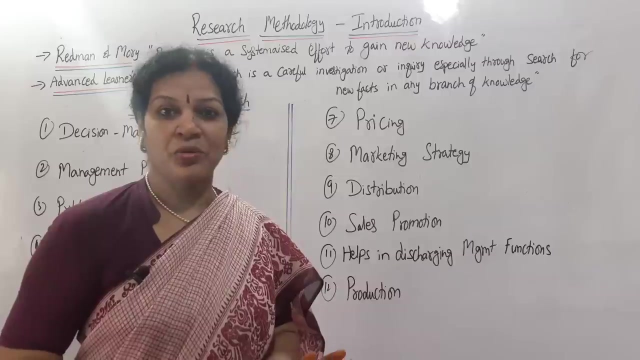 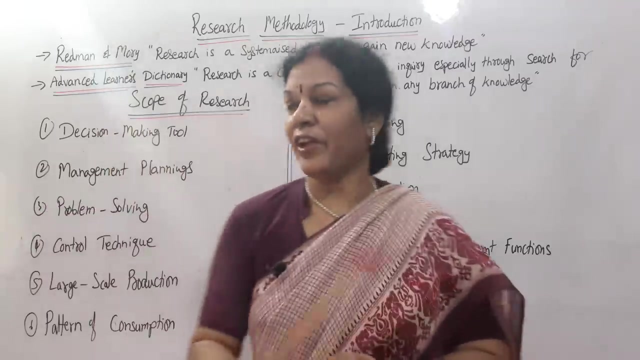 That area. what we are doing research is a careful investigation, Choosing any area, and we are doing careful investigation or inquiry, especially through search, Through search for new facts in any new area. This is also going to give you a vast knowledge and a good clarity about what is research Right. So in fact, you can say what is research means identifying a problem and 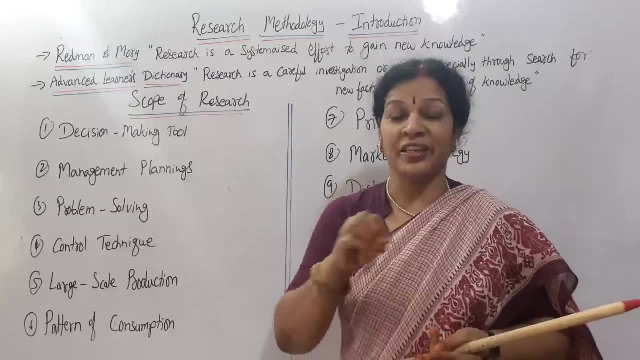 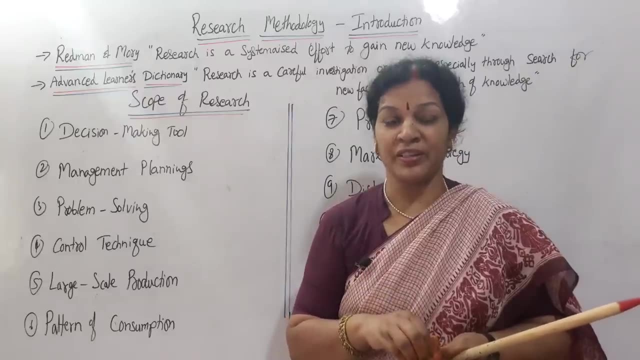 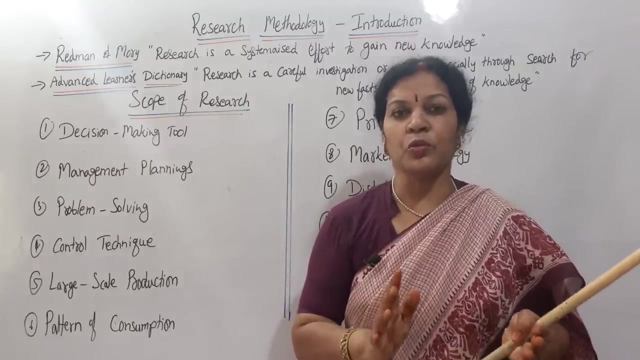 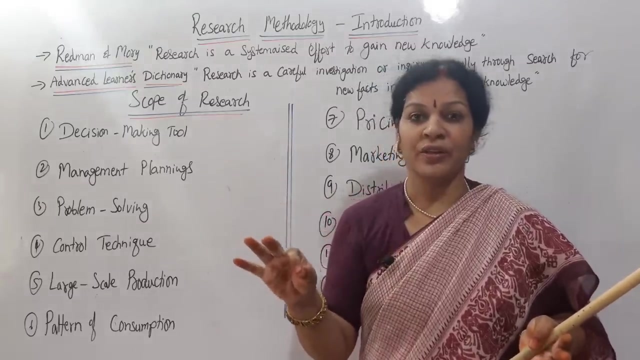 gaining the knowledge: Searching, searching and gaining the knowledge, and giving the alternatives and giving a conclusion, or you can say suggestions, findings. So these are all together, we can say it as a research. Now, related to the research methodology, let us see scope, Today's class scope, Where we can focus this research methodology, How we can focus it. That is scope of research methodology. This is the scope of research. Now, scope of research total: 12 points. 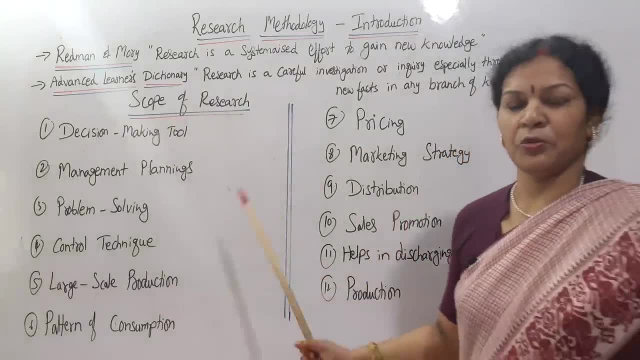 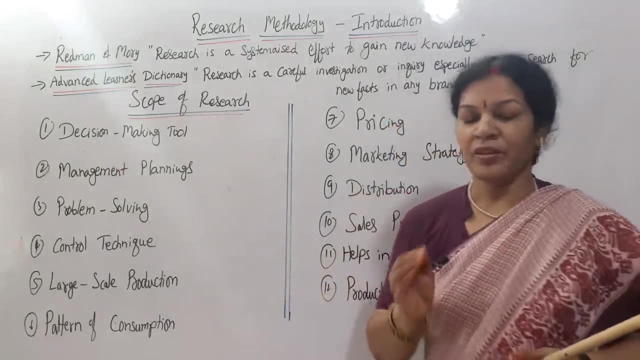 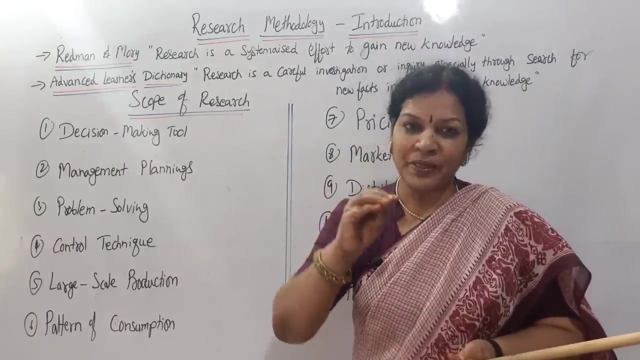 are there. Ok, These are the 12 points. If you understand 12 points, you will have a good understanding about research. First thing is the decision making tool. What is the research is going to give you? Research is going to give a detailed information about any particular problem. 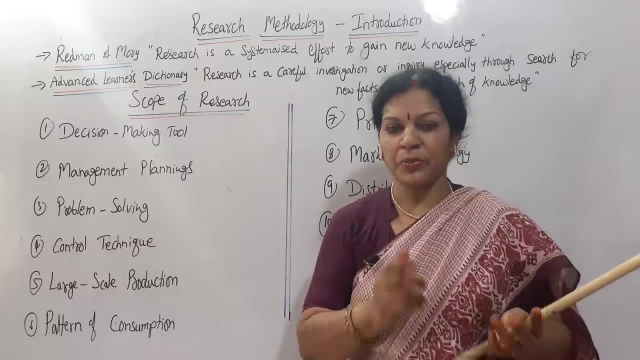 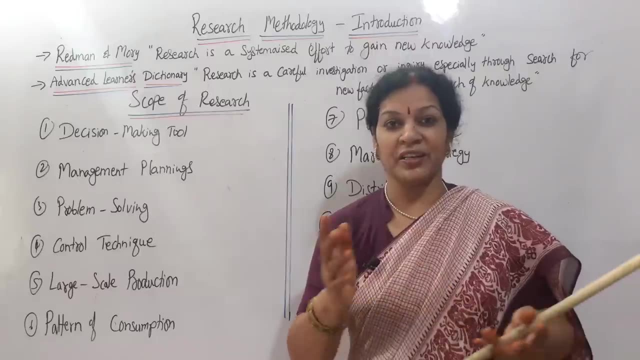 Any particular problem. Suppose say we have a problem of marketing. In marketing we have done any particular areas. See in store advertising or outdoor food, Political garbageывать, Healing Pub, Elmo hairstyle, Other physical barriers in R Want. Who are the? 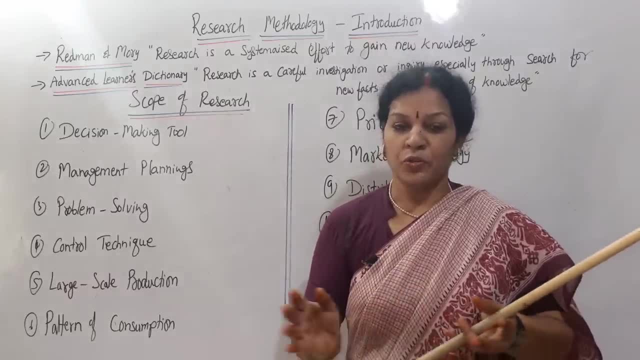 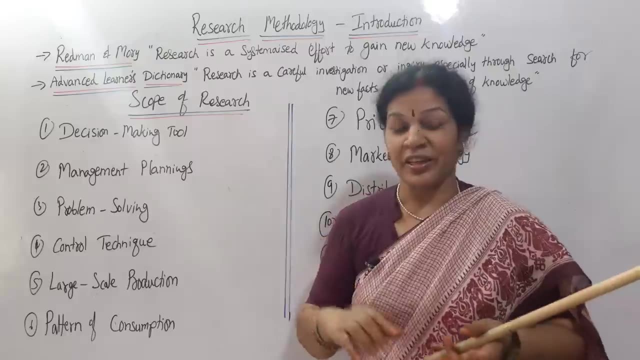 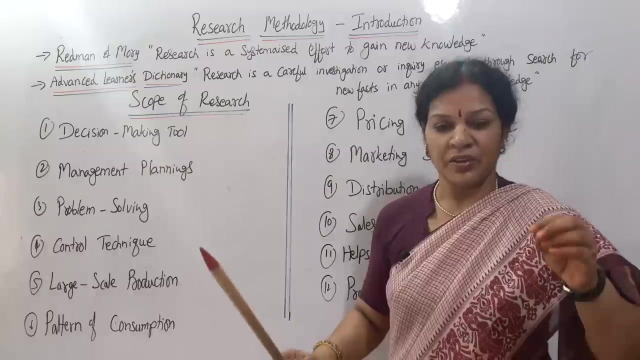 outside advertising. but this is one problem. so when we have done research, we get- we got a lot of depth knowledge. when we got a depth knowledge, then decision making is easy. so that is why research- we can say it as a decision making tool- if you have any problem, identify it, go for research and go for analysis, find. 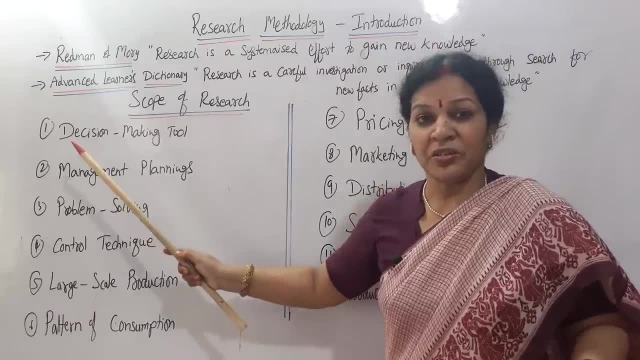 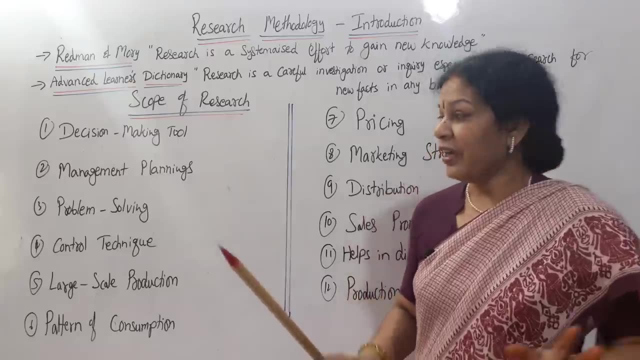 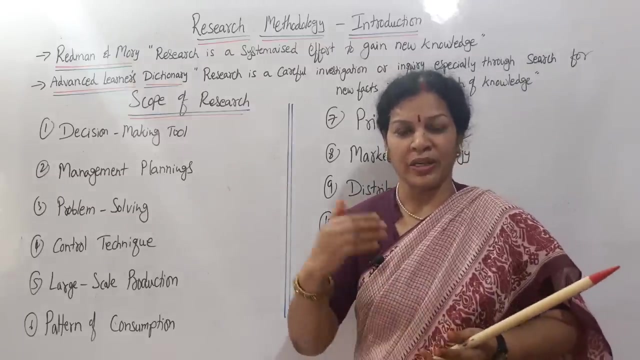 out, then you'll find alternatives. according to the, decision making is easy. that is why we say it as a research is a decision-making tool. okay, and in the same way, management plannings, when management want to take any kind of actions: forecasting and having ambitions, planning, implementation of planning, all. 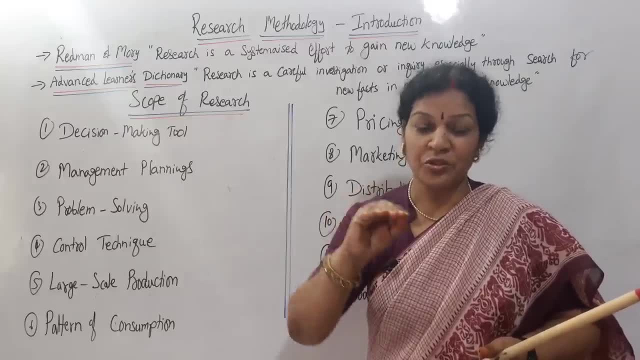 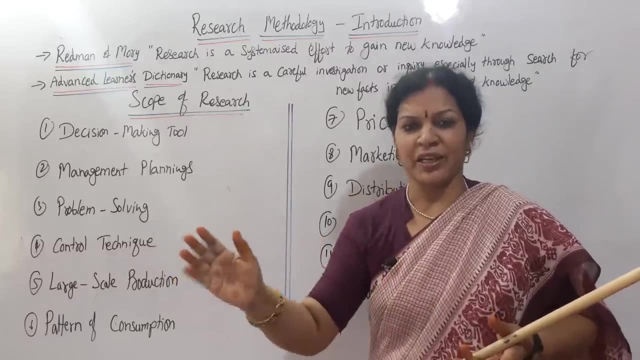 these things, research methodology. it is going to be very much helpful. research, research is going to be helpful. so how it is going to be helpful. any kind of problem when they are having, they can give us, they can throw the problem on someone, they can do the research and then 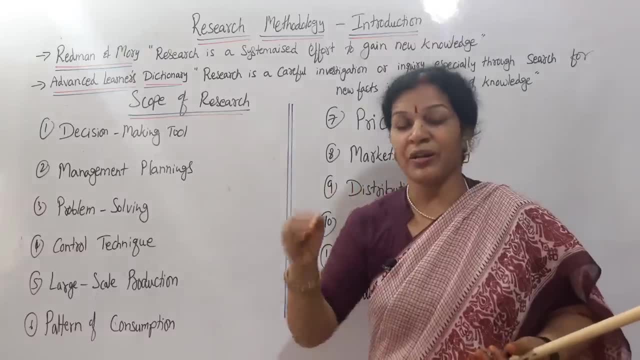 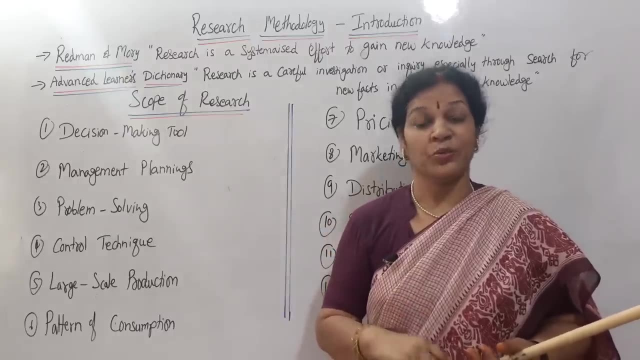 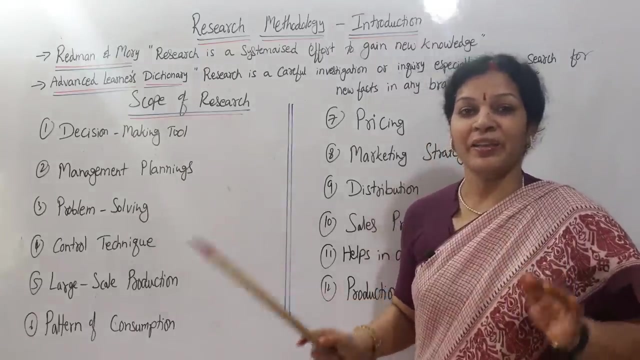 they'll come back. so, according to the solution, what they find it, they can take proper decisions, proper planning, especially for management. so they are depending on the research. this we can say. management is using this research for planning of their organization in the same way, problem-solving here. one. 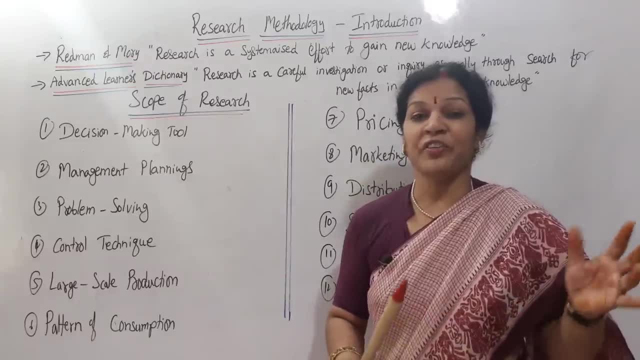 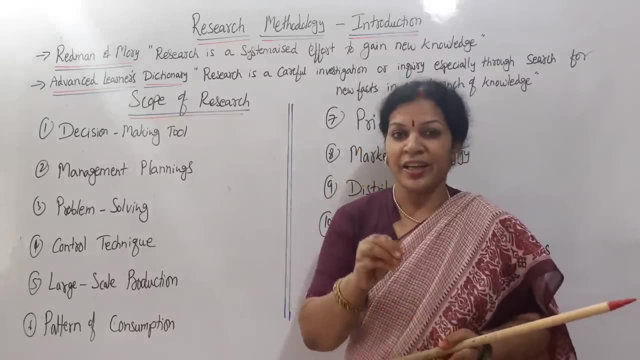 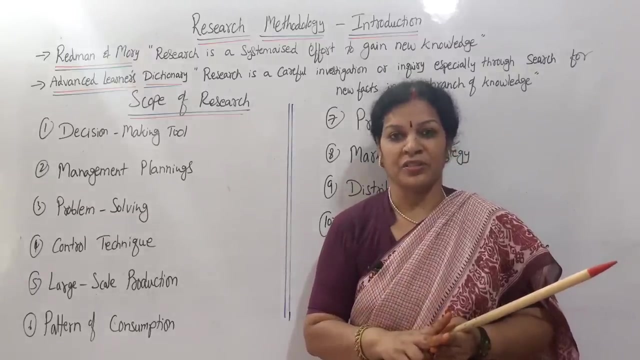 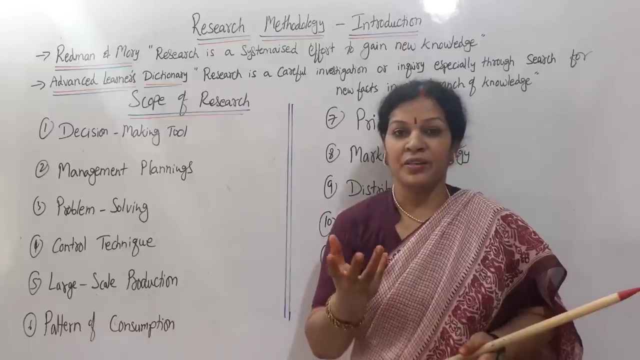 thing you must remember: simply blind, you cannot identify any problem, exactly what the organization is taking, what the organization is facing. that kind of problems only have to identify, identifying the problem and finding out the solutions. sometimes the problem is not there, but still you are assuming and you are. you are assuming and you are. 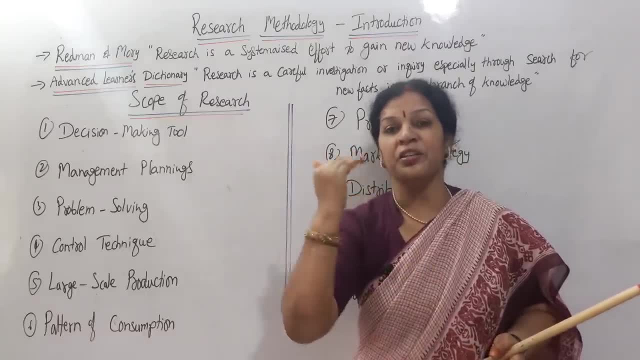 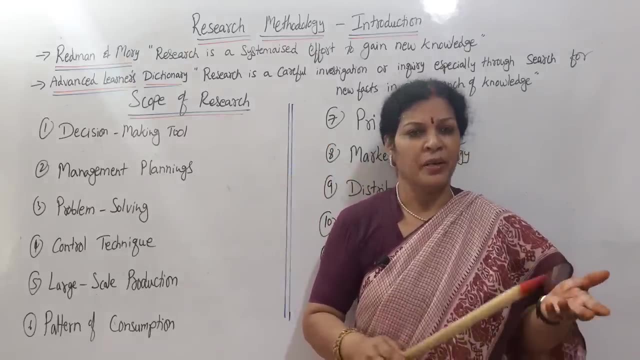 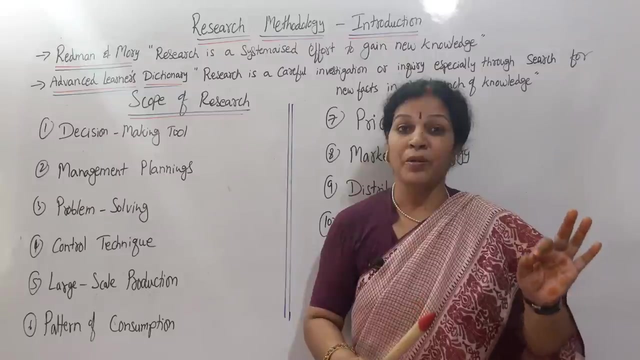 estimating or you are doing some kind of research on related to the problem which is going to occur in the future of your organization. this is a very important part of our organization in future so that kind of problems we can identify, present problem or future problem, just forecasting. according to that you can identify problem, solution is possible through. 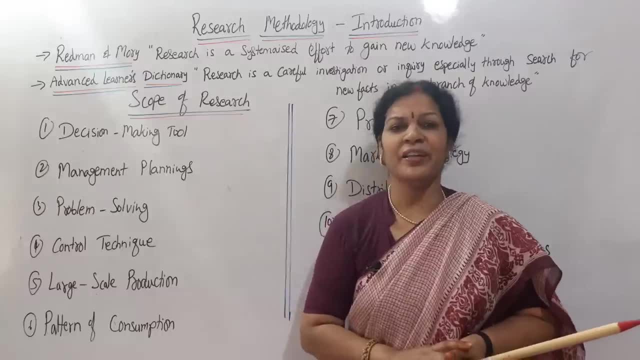 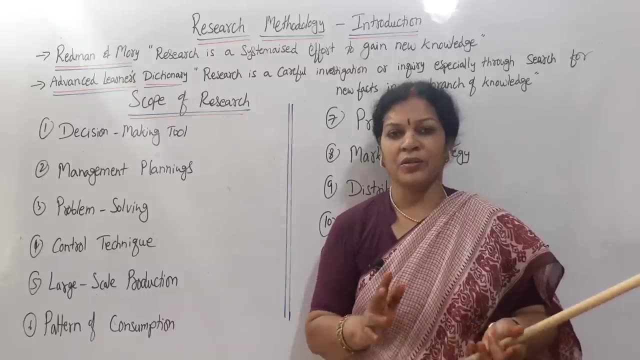 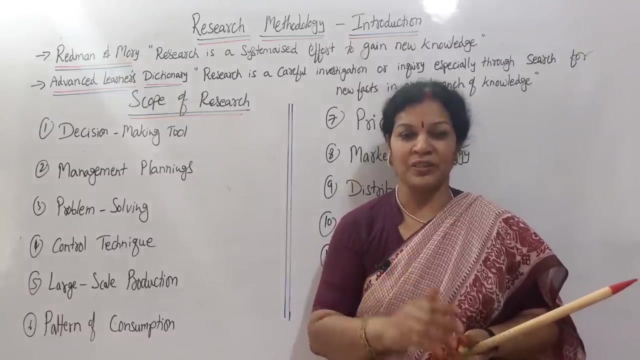 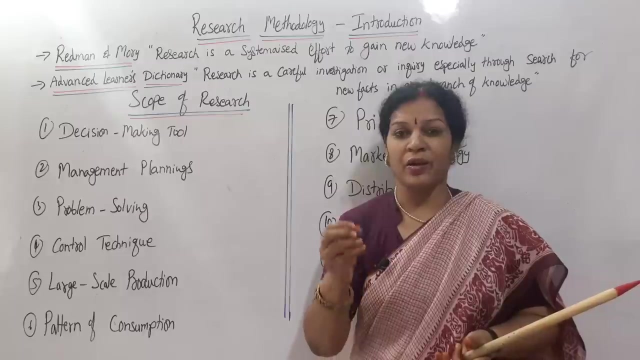 a research example i'll tell you. we had a very big crisis once upon a time, especially in finance area. there was a lot of economic problem and also recession during that period. some research was went then. according to the research we just identified where it is the problem is lying and how we can find out it. all these things through research. we. 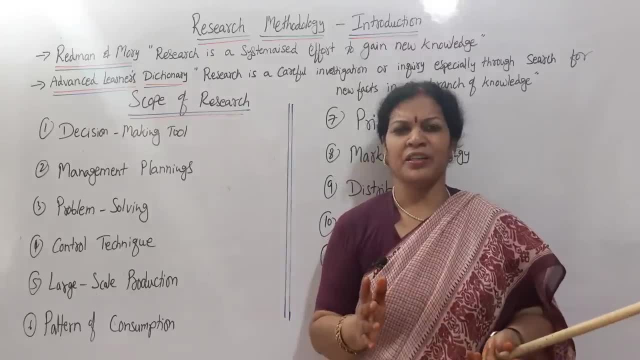 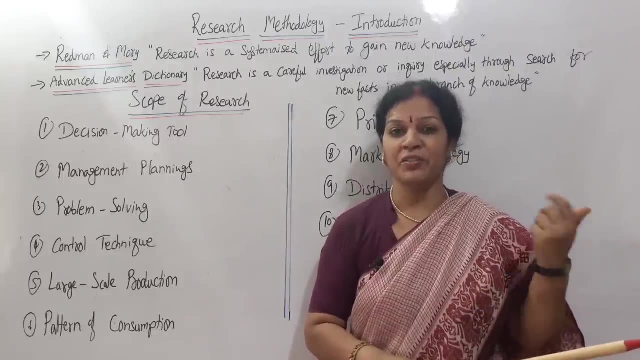 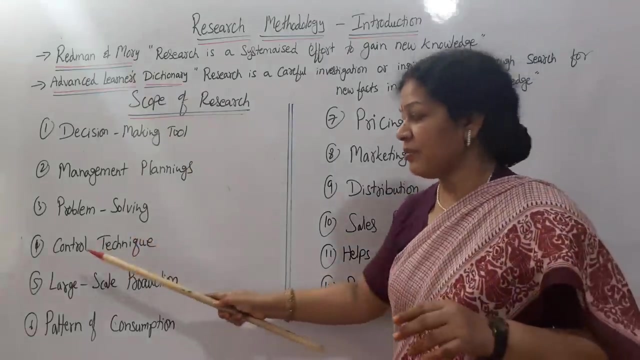 have done. any area you can take- marketing area you can take or otherwise, hr area, finance area, any area you can just go ahead identifying the problem and giving a solution. that is about problem solving, which will be very much helpful through research only and in the semi-control technique. you know that we have a lot of problems like how we can control it. 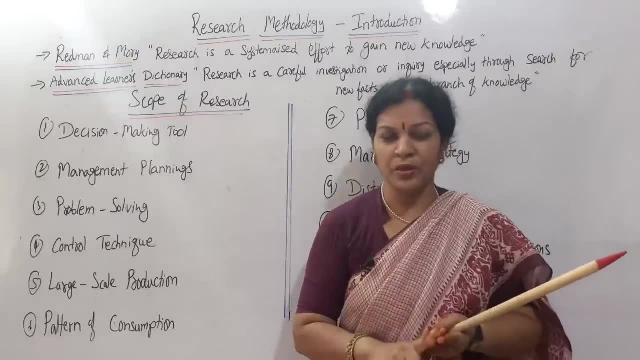 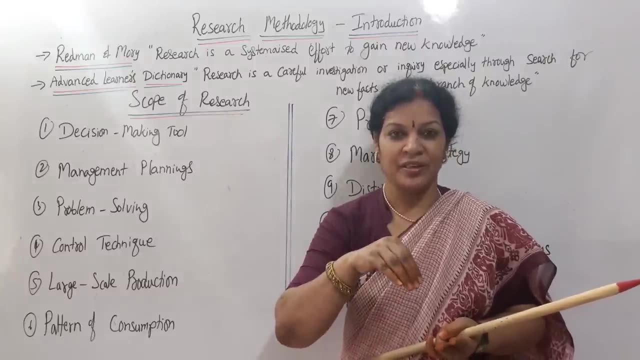 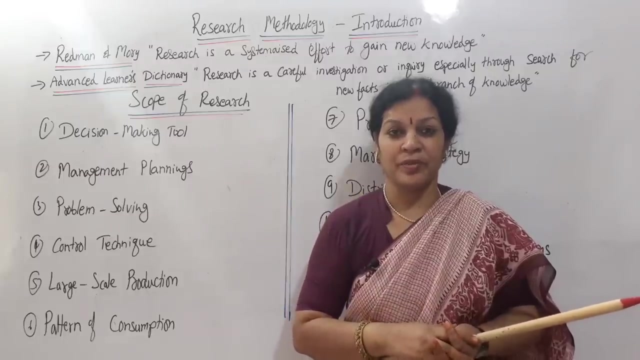 example, if we take we wanted to control the organization, how we can control, if we have good idea about how the organization is running and what kind of methodology we are following. how is the finance area? and let us focus on the customer. how is the customer behavior? how is the marketing? 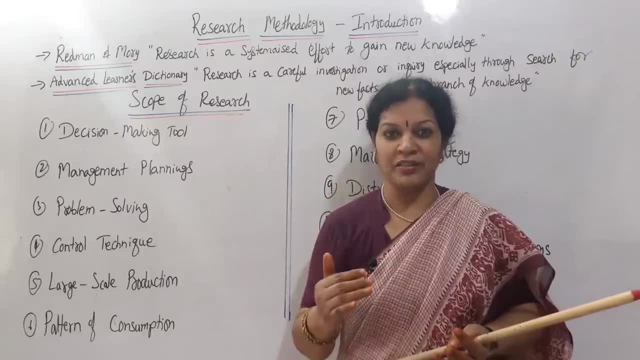 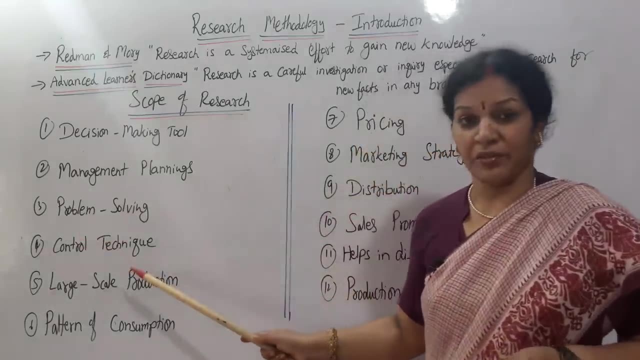 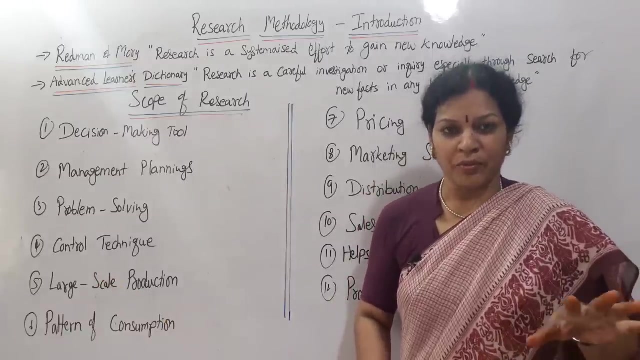 strategy. is it increasing demand? is it increasing demand? is it increasing demand? is it increasing increasing demand? supply and production availability. so all these things we can just consider under this control technique. we can control it. say something is not under control, then just do the research. then what? what are the main reasons for uncontrollability? 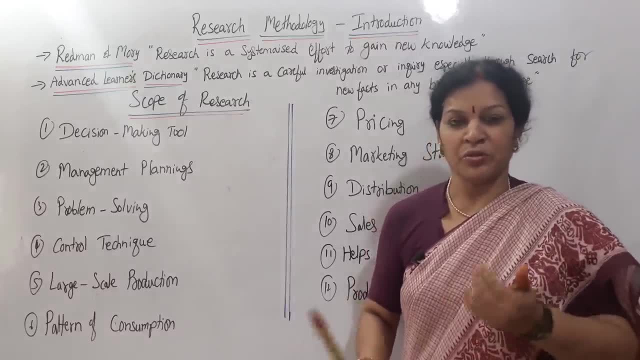 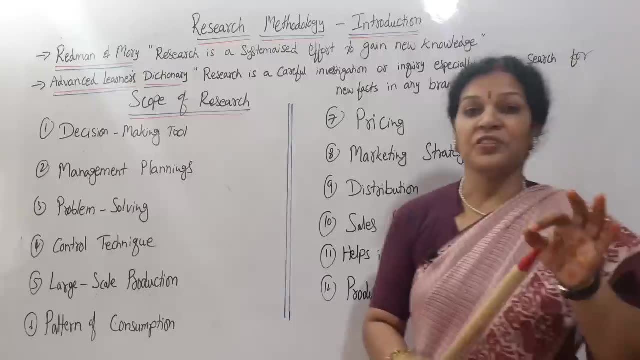 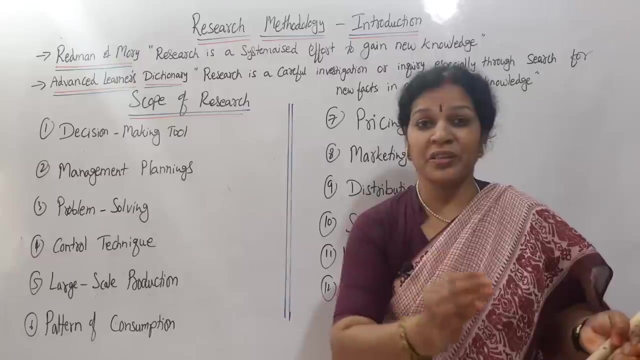 find out the reasons and find out the solutions and also go for the alternatives. in that way you can go for controlling technique okay. in the semi large scale production research is very much useful. small scale industries and also large scale. small scale according to the requirement. you can do the research for large scale- much useful because you can't take the 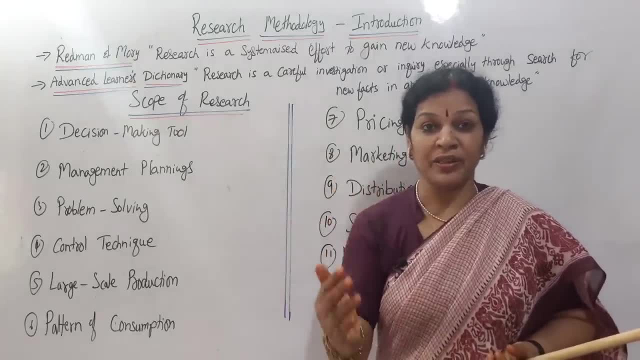 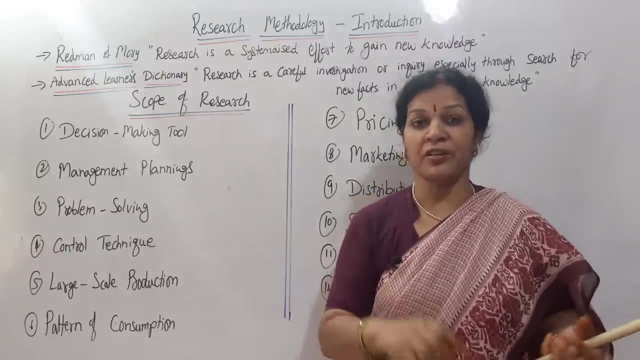 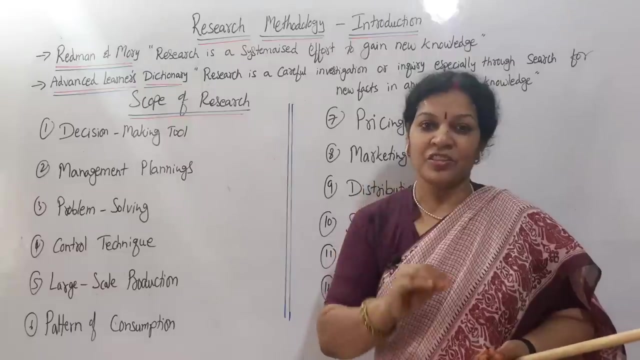 decisions blindly. you can't go ahead simply because you need to have some understanding. large scale production: i'm going to produce it, i'm focusing on a large scale. then before going to that, i must do some research. research or identifying the problem and finding out the solution. all these things can be given to 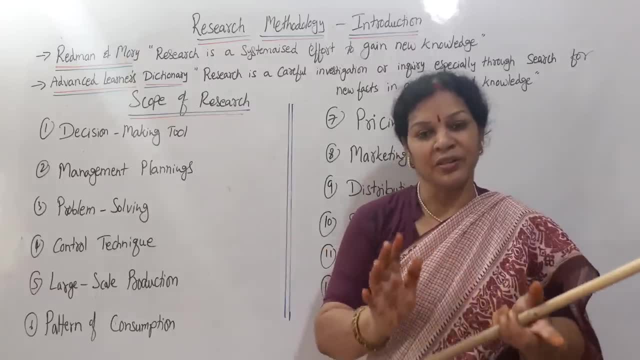 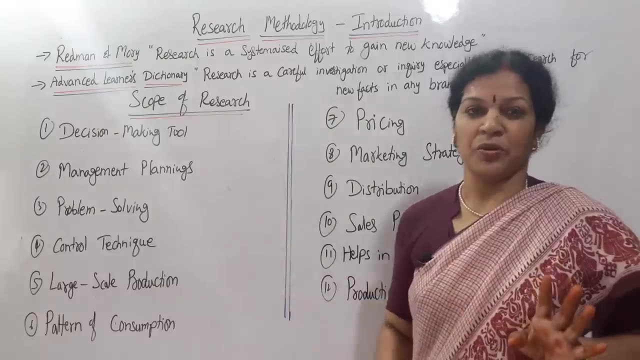 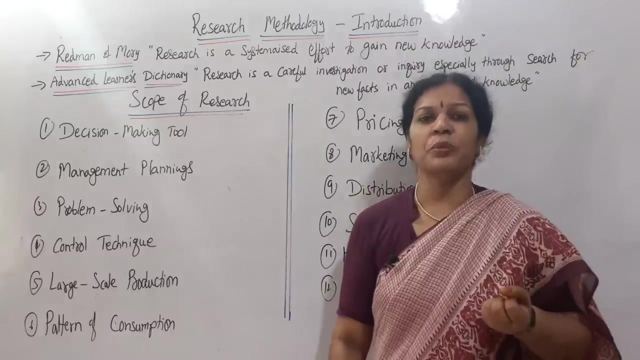 the expert and whatever outcome we get according to that will study and then we can go for the large scale production. for that purpose it is much useful research in the same way, pattern of consumption. pattern of consumption means generally the consumer behavior it comes. every consumer is having different kind of taste at present. 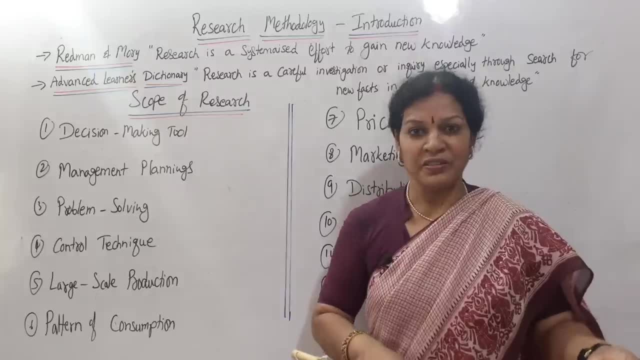 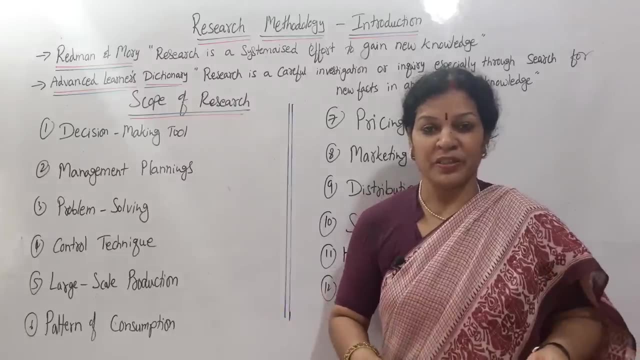 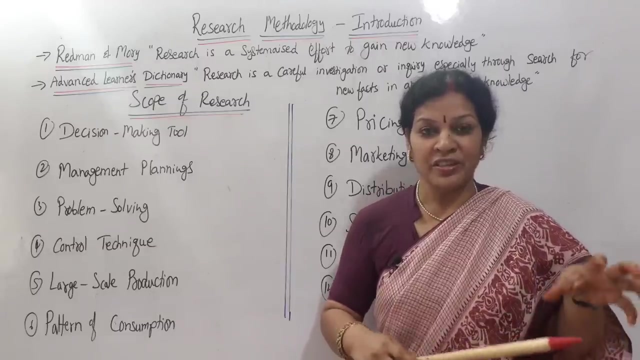 there's a lot of demand. tomorrow may not, our present demand is not there, but tomorrow we can increase the demand. how we can increase what is the taste of the consumer, what he is expecting. where we can make the changes of the product. how we can promote the product. studying about the. 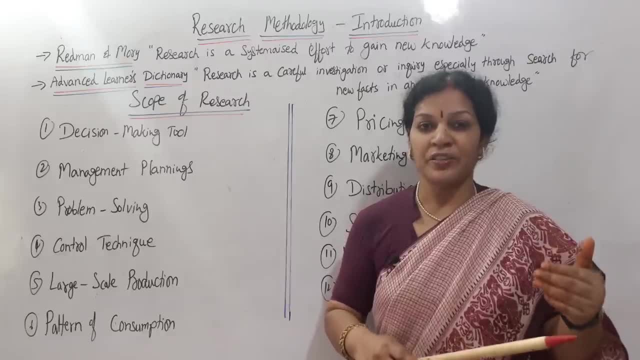 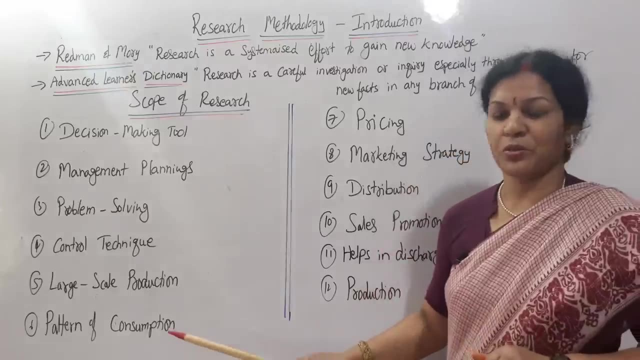 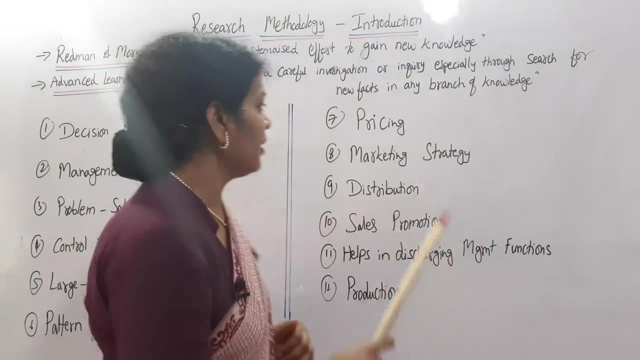 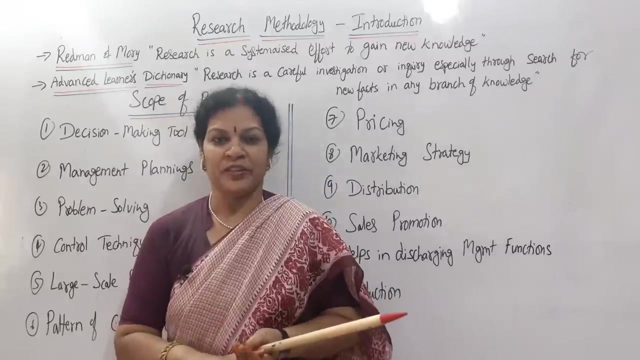 consumer and his behavior and his, his taste, and also marketing study. all these things together, we can just go ahead in this pattern of consumption. if you know this, we can plan accordingly. and not only that, there are a few more things that is. another thing is that pricing very important concept in marketing especially? 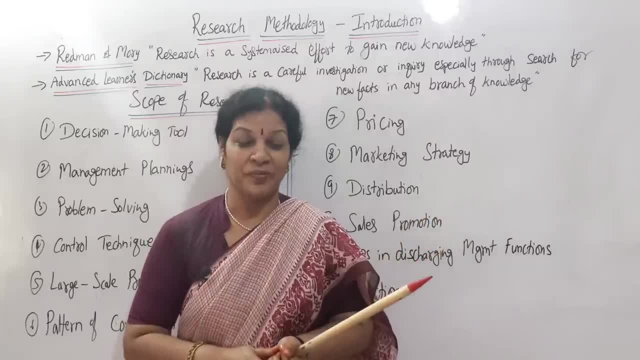 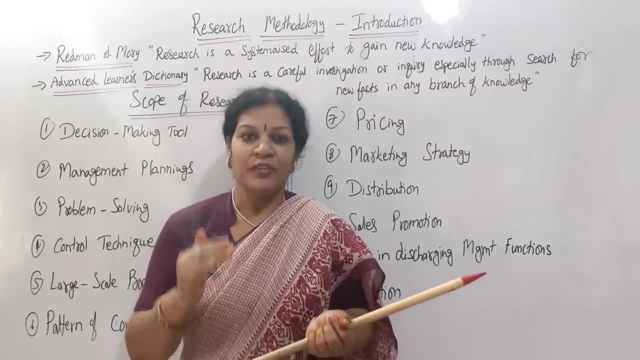 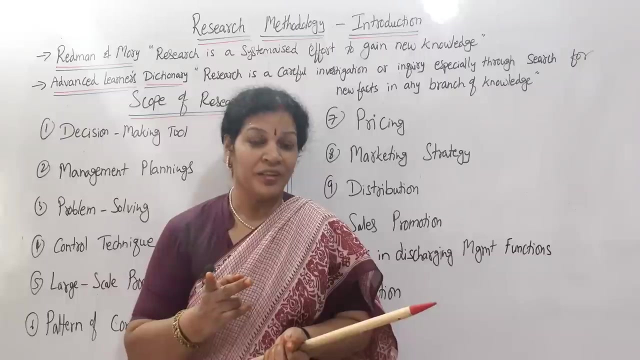 when you decide that price should be this much, that is going to make the impact on the mindset of the consumer. say, if you are increasing the price, sometimes consumer may not accept it where there is no alternative for that product. if you increase the price also, there is no other solution for the. consumer. he has to buy and he has to consume your product. there is no other alternative, like sometimes, if you decrease a little bit of price which is less than the other competitors, then definitely it makes a lot of difference. it may or may not so that price fixing strategies are. 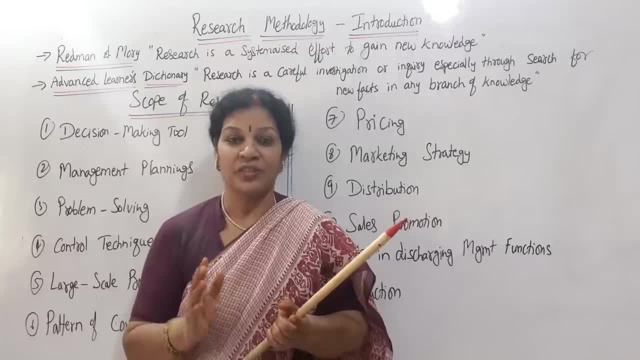 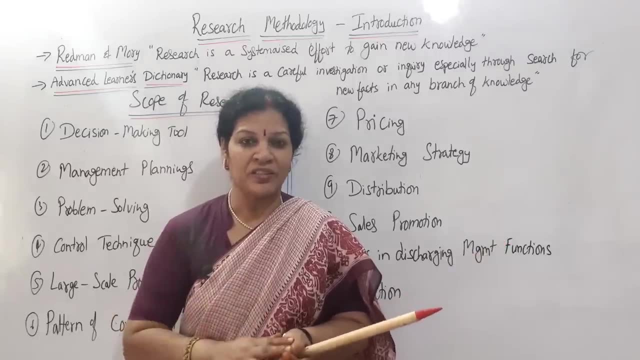 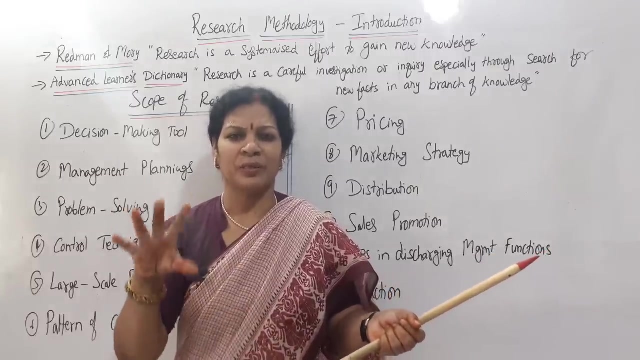 possible through research. through research, you can just find out. so at what rate we can fix and what are the alternative products are available in the market. what is their pricing strategy? what is the quality of their product and how is our product? what should be the price? like? we can go some research then. 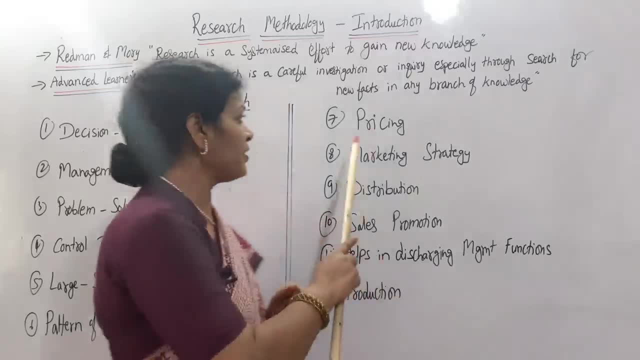 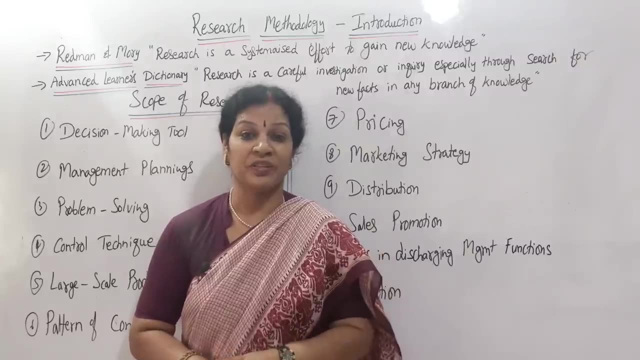 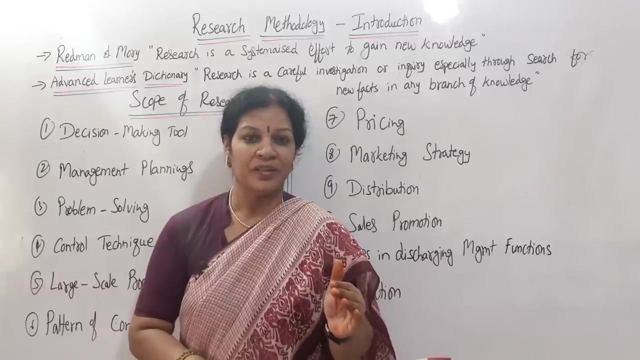 after that you can take decisions right. so that's about pricing and marketing strategy. marketing strategy also how we have to launch the product, when we have to launch the product, where we can launch the product, how should be our strategy, how to attract the customer and all these things which comes under the marketing. 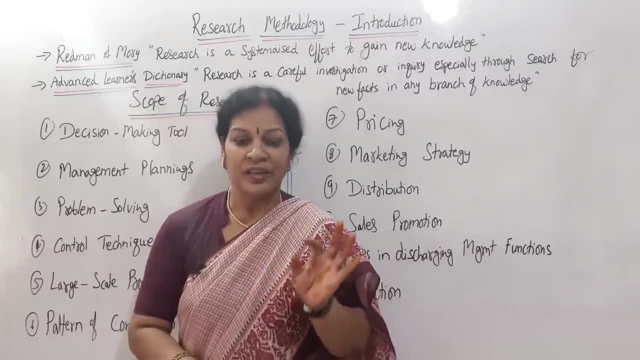 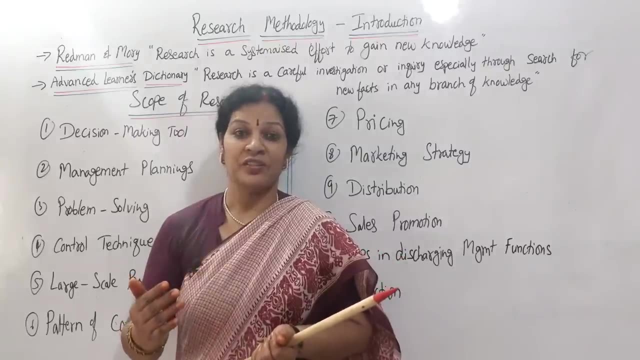 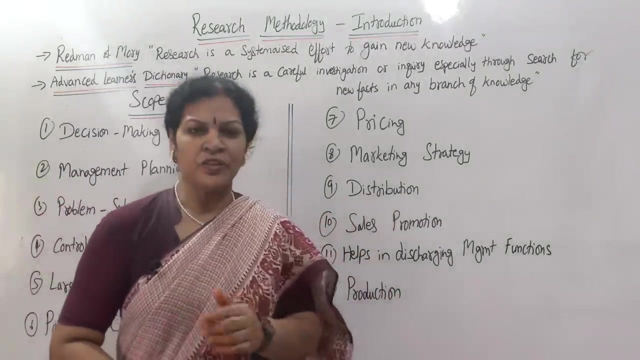 strategies. if you do a small research related to that particular aspect, then it will be easy for us to take decisions and proceed for the marketing strategies. so for that research is useful in the same distribution. distribution means once the product is ready until the product reaches to the 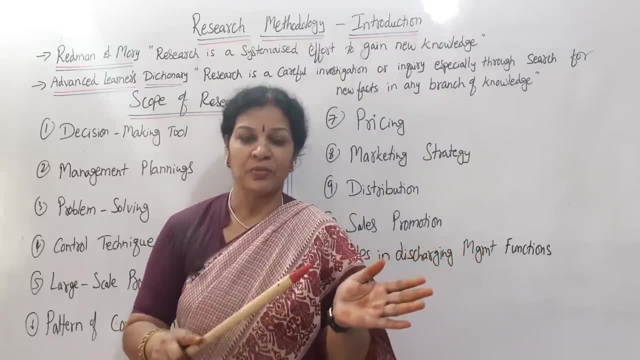 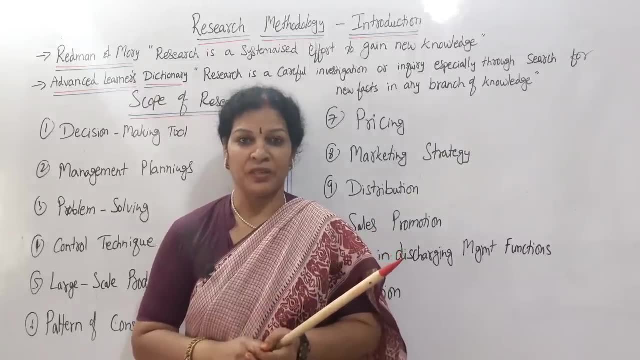 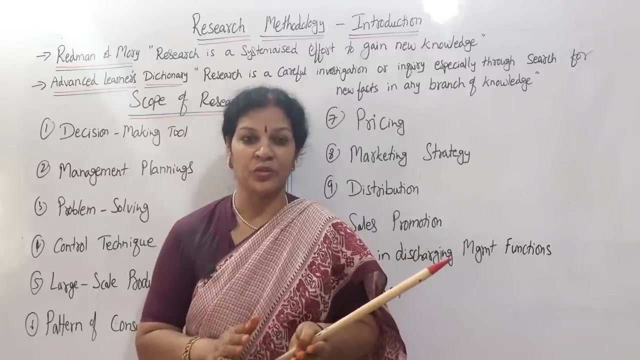 consumer, the channel, everything process. we call it as a channel distribution. so channel distribution, how we can do which one is the best way, how we can reach the consumer quickly and with less cost, which channel is going to be workout, so that channel distribution also, we can just go for research then. 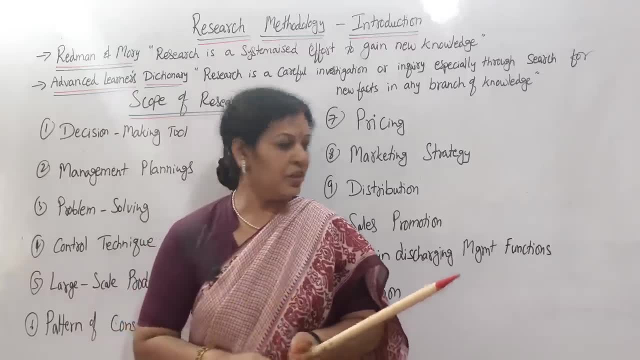 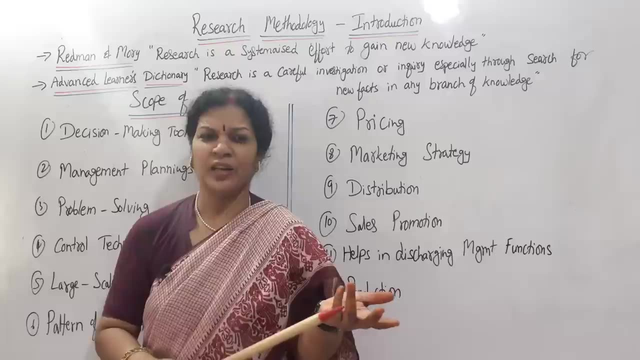 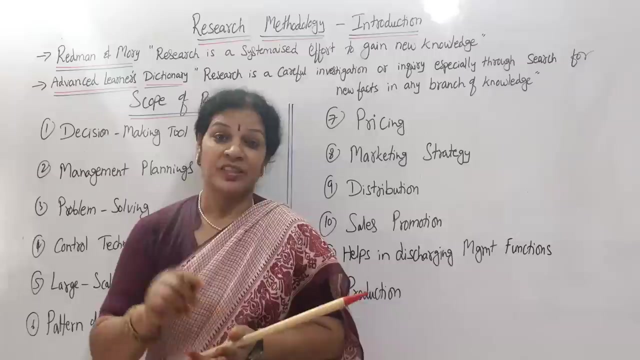 according to the outcome, we can take the decisions right. in the same way, sales promotion, sales. we wanted to promote it. how we can increase the sales: there are many strategies. if you go for marketing subject, you will come to know how we can increase the sales. sales promotion is very 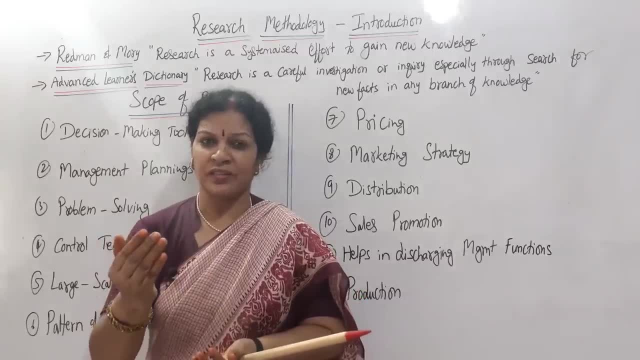 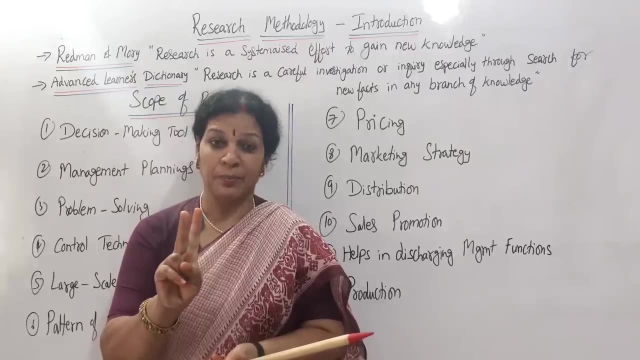 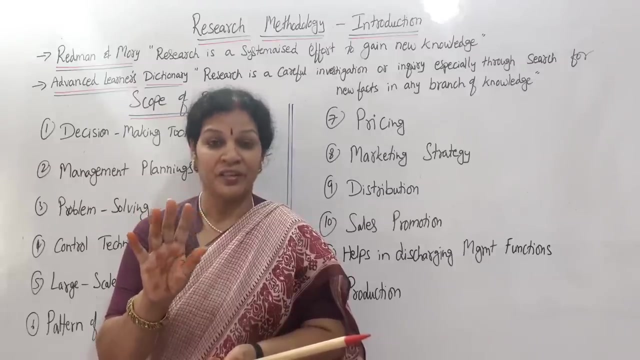 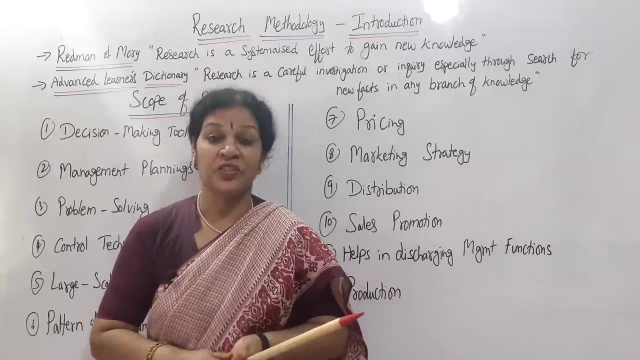 much important. so how we can increase the sales, sales. so i'll just give you an idea: maybe quality of the product you have to improve, or apply the new technology or otherwise. pricing strategy and packing strategy and distribution of channel, like various strategies, are there to increase the sales, promote the sales, which one is better and how we have to proceed it. 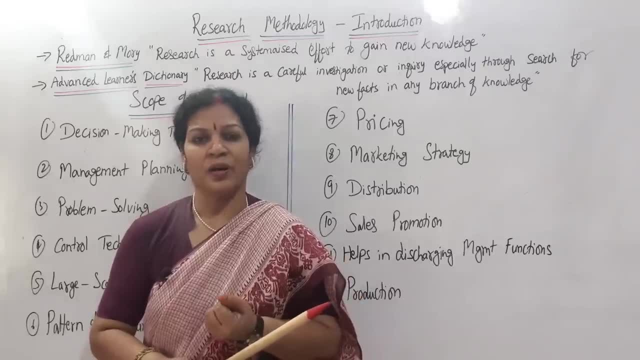 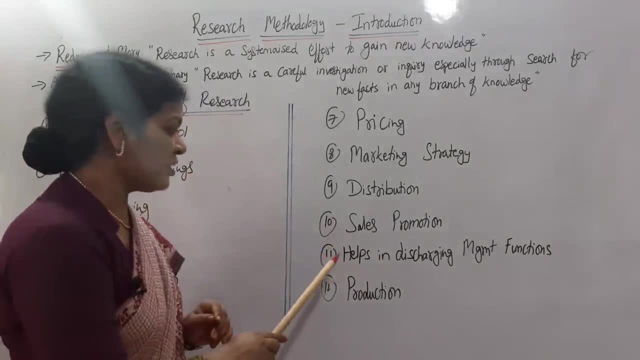 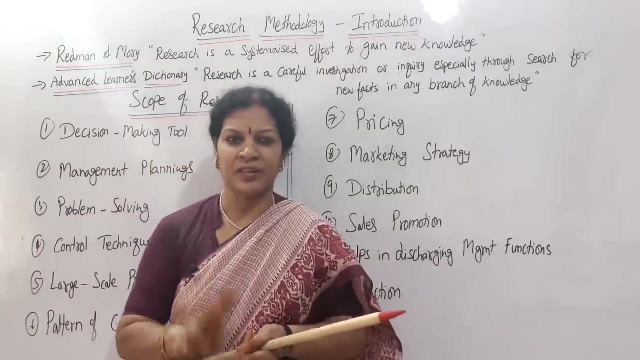 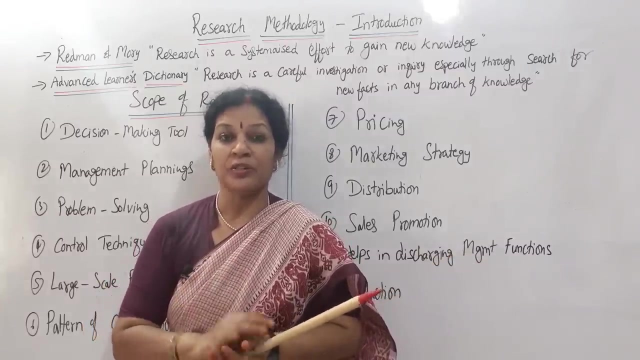 do the research, then, as per the outcome, we can just go ahead. so that will be useful or beneficial for any organization. in the same way, it helps in discharging management functions. you know that management functions we have studied: planning, organizing, controlling, staffing. okay, so all these functions. when management want to continue their functions properly, then research is going to be. 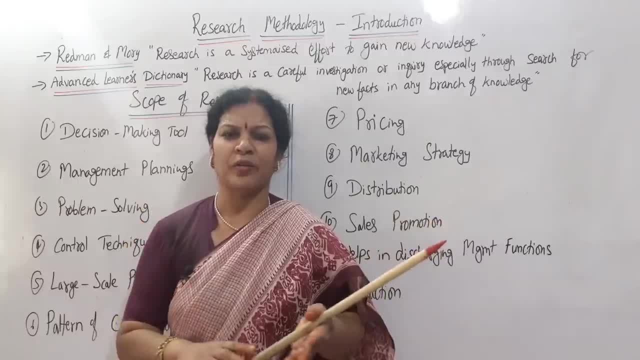 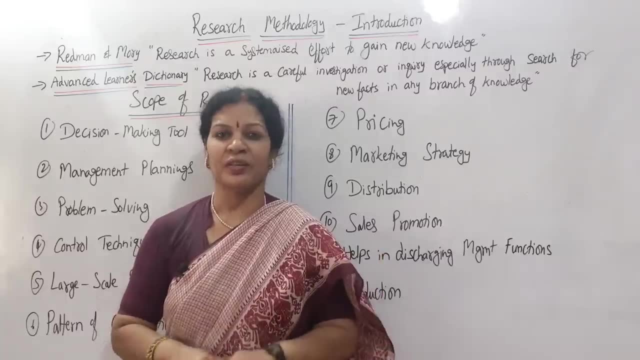 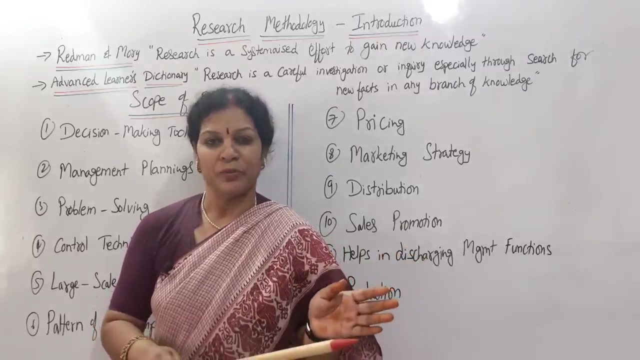 very much helpful. any problem arises, as anywhere, then automatically the management is focusing on that particular problem, depending on this research, and then we come to one conclusion or take a decision. so for management to fulfill the management functions it is going to be helpful in the same way. last point, production. 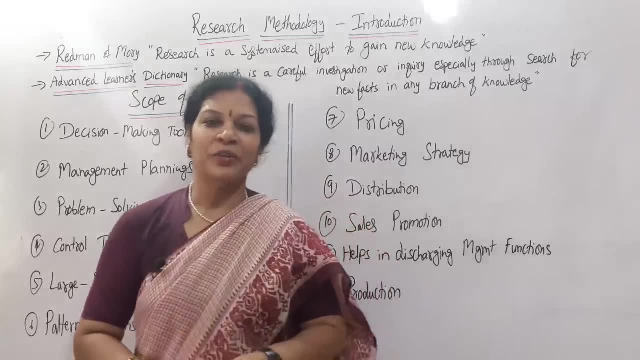 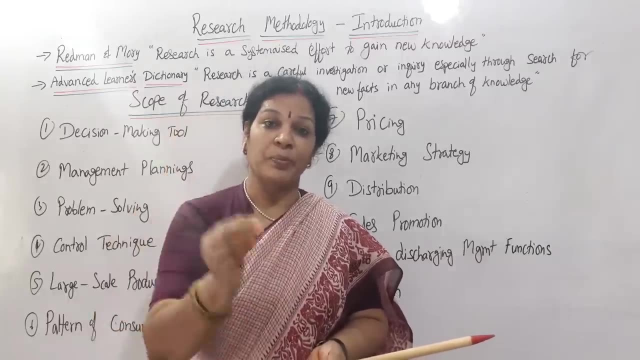 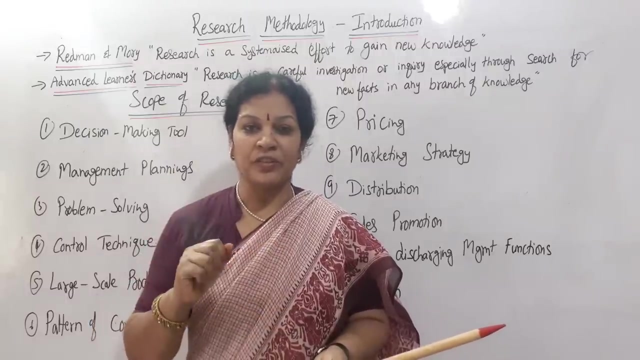 very much important: production. how do we do the production? according to the demand: if demand is there, will focus on the more production. if demand is less, we have to decrease the production. so this strategy, also production study- this is one thing- as per the demand, production increasing or decreasing. 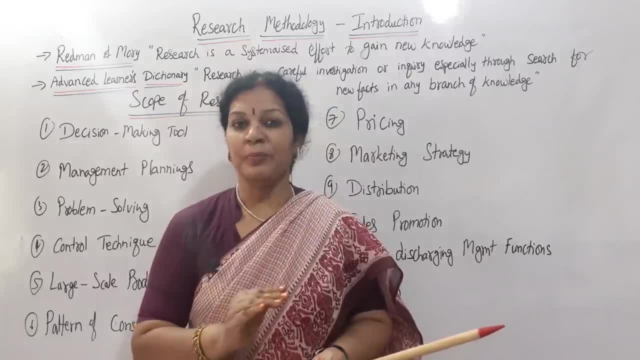 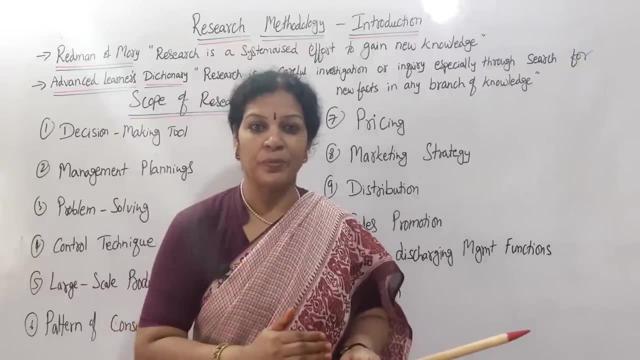 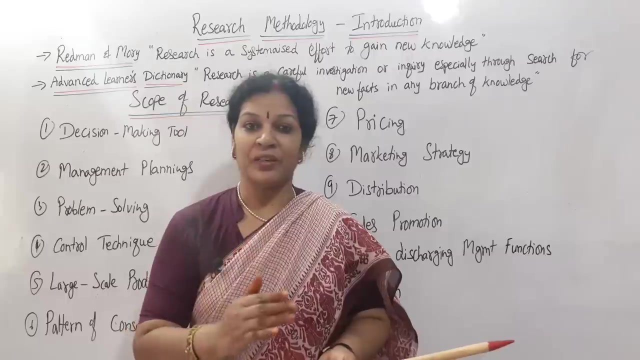 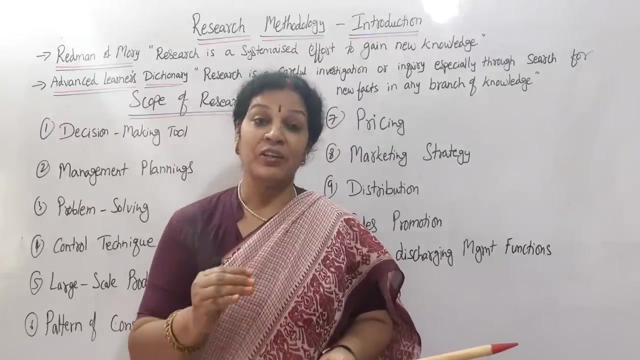 and another thing is that production depends production cost. let's focus on the production cost, the production cost. if you decrease the production cost, what happens automatically? price. we can decrease it. where we can cut the, where we can cut down the expenses, how we can decrease the production cost so that we can give. we can give our product to the consumers at the best price. 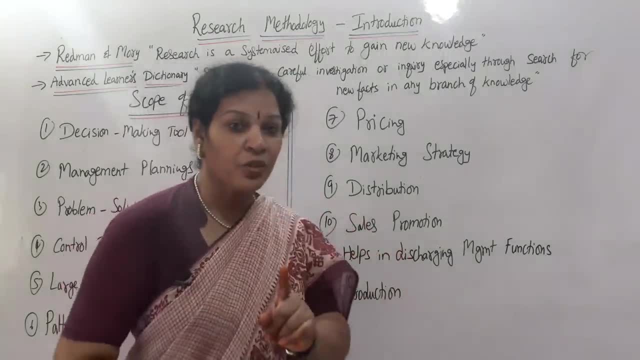 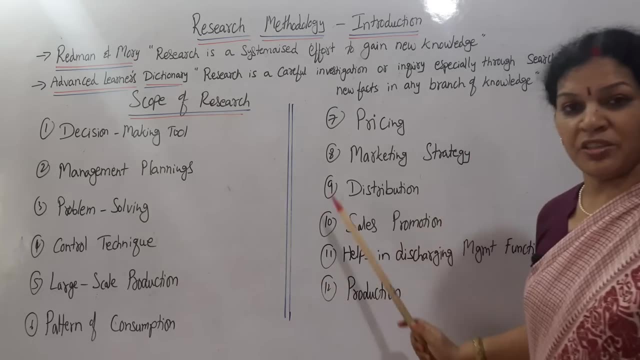 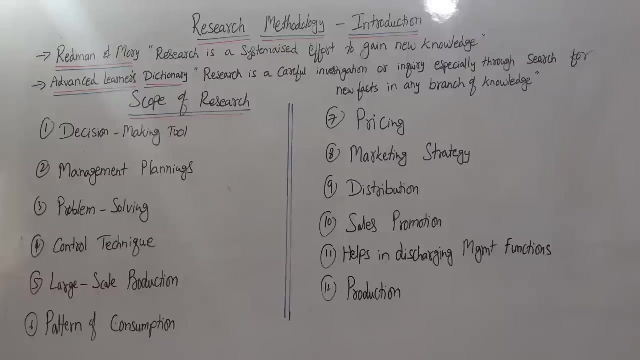 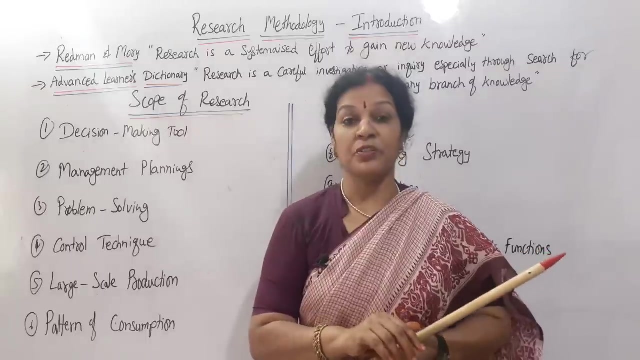 in that way, you can just focus on the production through research. okay, so these are the main areas where we can focus on the research. the such scope is there there in all these areas. take a screenshot or note down. in the coming few classes we'll be discussing about research methodology- very important. 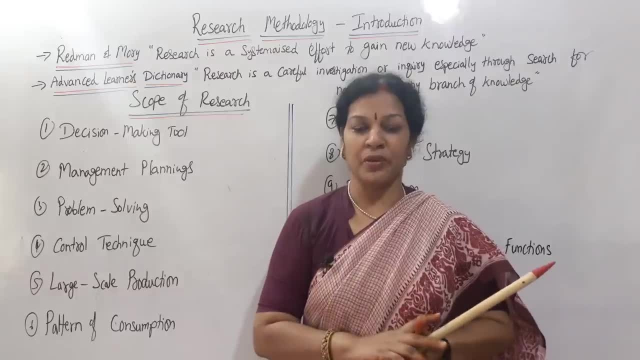 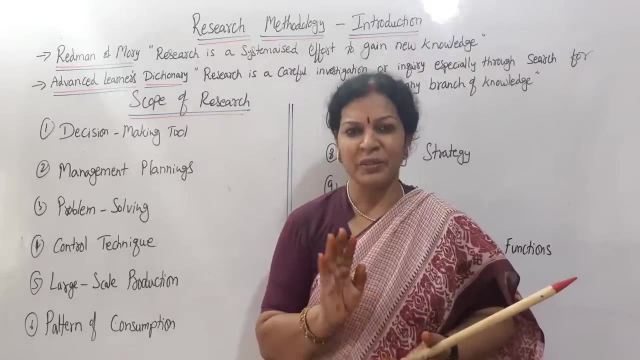 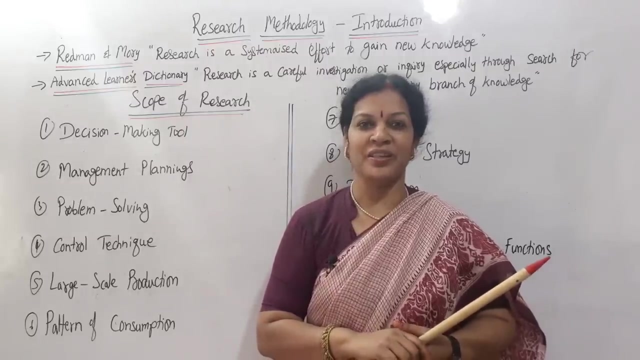 theory parts theory theory examination point of view. I will take a few important topics. after that we'll go to the problems. by the way, feeling comfortable, somewhat understood about the research methodology, if you understand, please write it in the comment box. I wanted to see your expressions, I wanted to hear from you and how you're feeling it. anything I'm 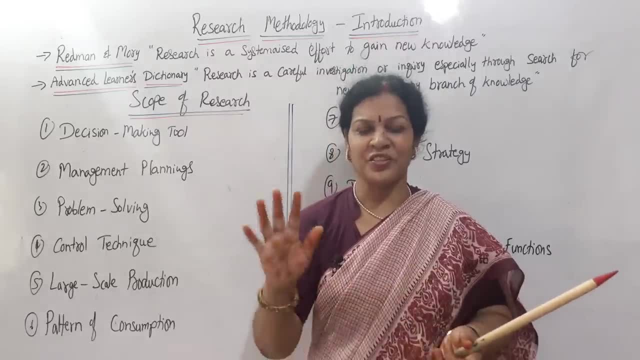 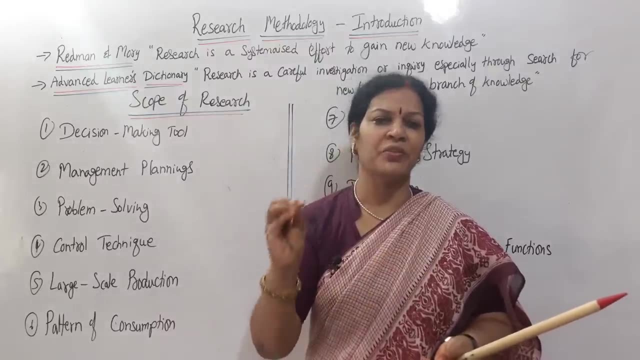 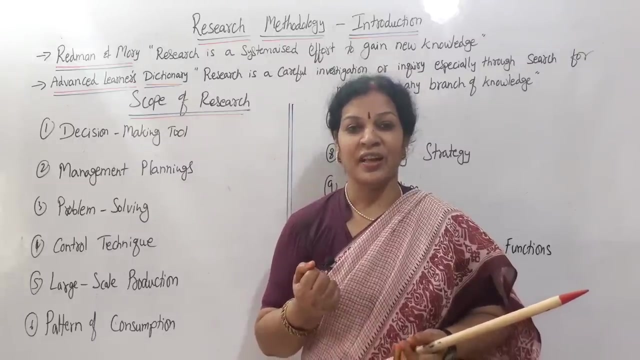 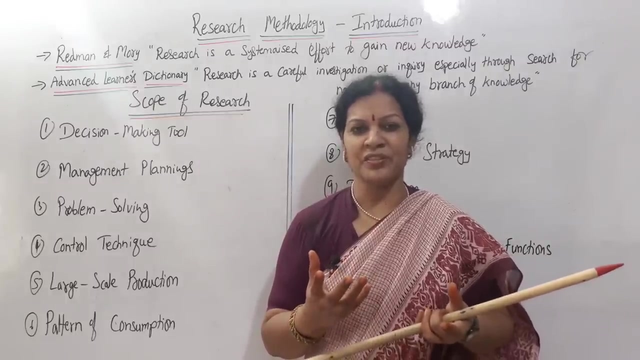 waiting for your comments. and, by the way, all these lectures, many subjects already prepared and uploaded, all these lectures are free of cost to everyone. every student can use it without any hesitation, gain the knowledge, utilize it and come up in your life. this is my ambition. let us support, let us work out together, both of us, so that it will be beneficial. 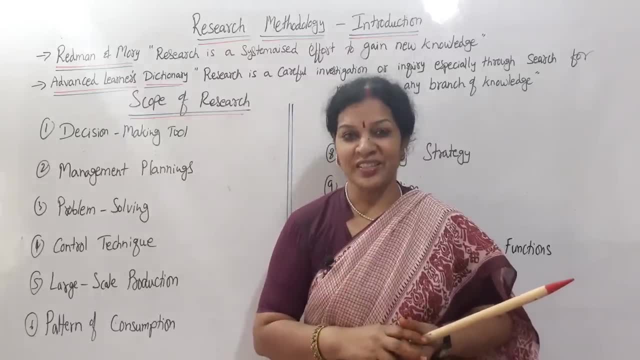 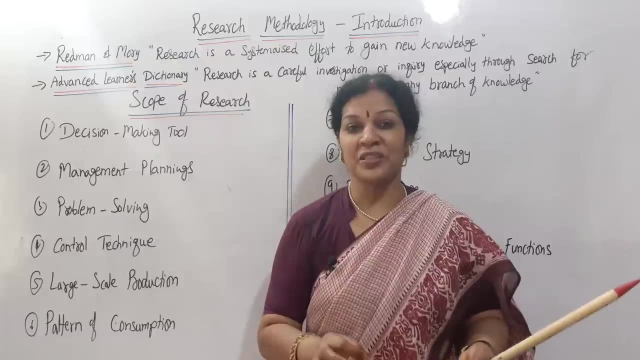 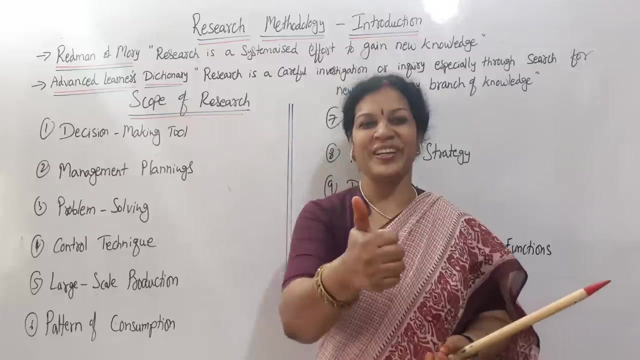 for your career point of view. stay connected, don't forget to share this videos with your near and dear and practice well throughout your semester. before exams, just revise it. remember this, funda, and study well. have a bright career, good luck.